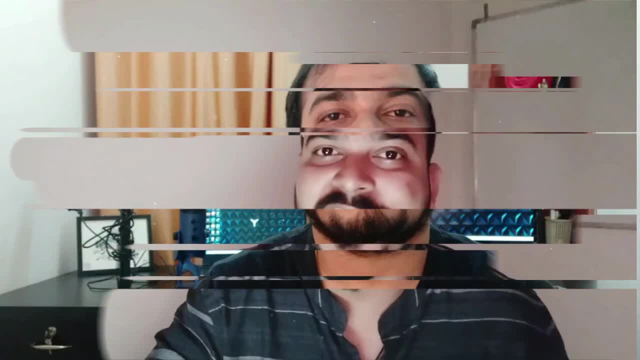 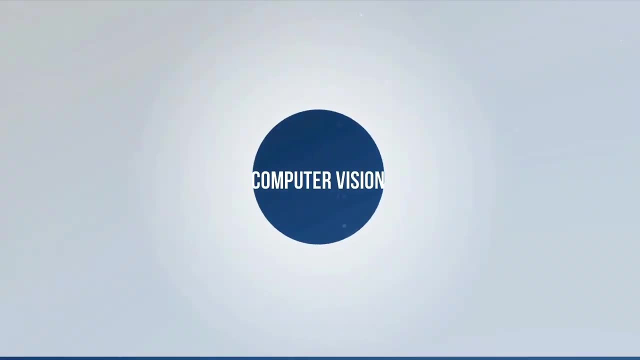 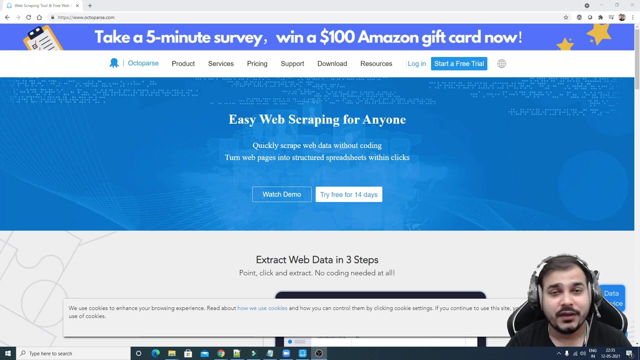 Hello all my name is Krushnak and welcome to my YouTube channel. So, guys, today, in this particular video, we are going to see this amazing tool which is called as Octoparse, and this particular tool will actually help you to web scrap in an amazing manner. Now, 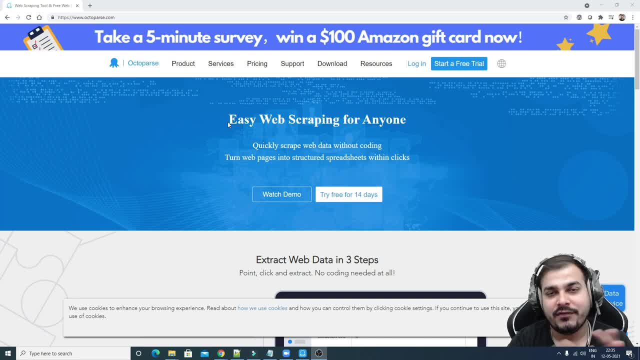 you can use this particular tool for web scrapping in any different kind of websites, and I'll try to show you various examples. We'll try to scrap an Amazon web page and we'll try to see how the products, along with the pagination, will also get scrapped. Now the first step. 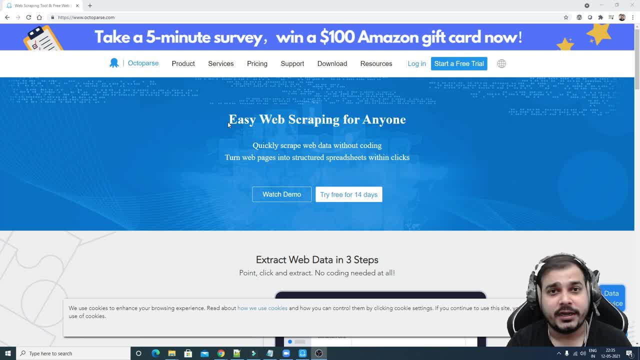 is basically to download this particular tool and try to install it. Let me show you the steps with respect to how you can actually go ahead and download it, And then we will try to take an example with respect to an Amazon web page. We can also take an example of Flipkart. We can also take examples with respect to eBay. 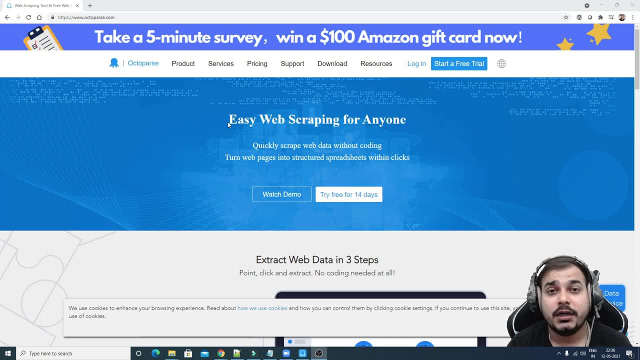 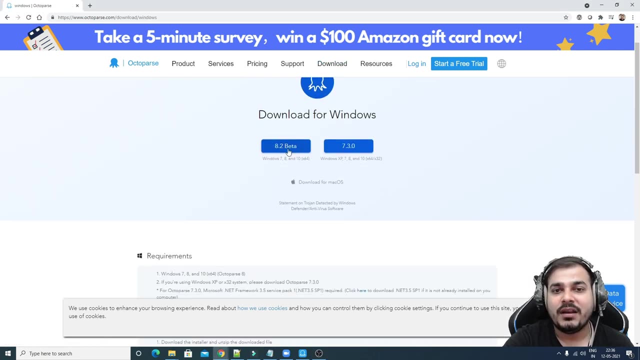 various, different, different sites, And one amazing thing about this particular tool is that this tool actually provides you multiple templates based on different, different e-commerce sites. I'll show you that specific example also. So let's proceed and let's go and download it. For downloading, just click on download and here you have one beta version and one. 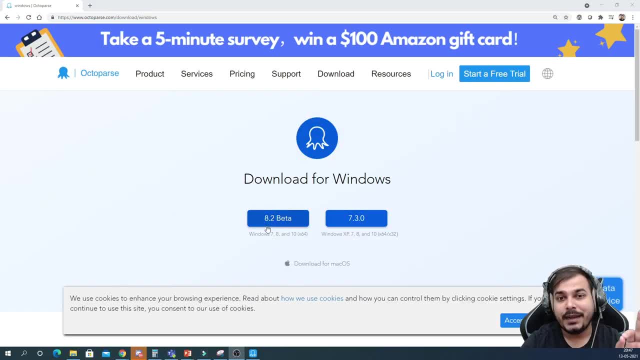 7.3.0.. So, guys, out of these two versions, that is, the 8.2 beta and 7.3.0.. So, guys, out of these two versions, that is, the 8.2 beta and 7.3.0.. Try to download the 8.2 beta version. 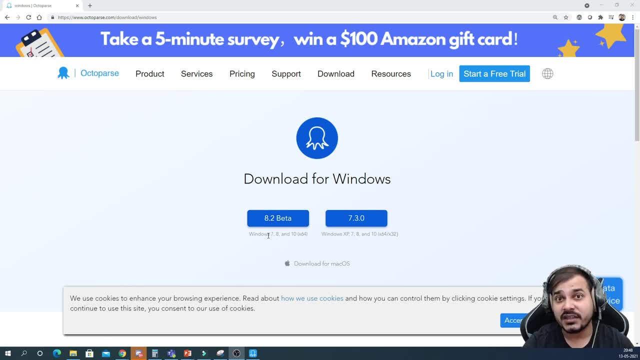 because it has some more additional functionalities. It is quite fast and it also has a very important functionality which is called as auto detection. So in order to download this particular version setup file, just click over here, and here you'll be able to see that the file will get. 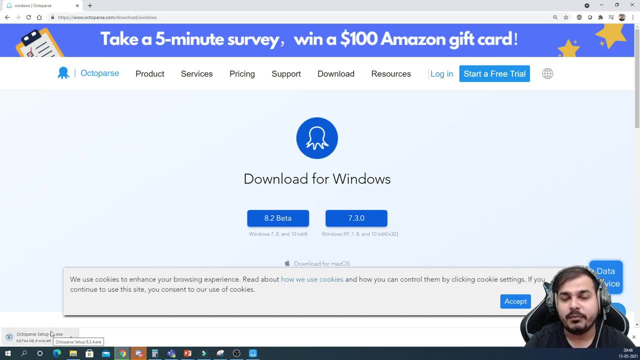 downloaded, So probably you have to wait for some time. It depends completely on your internet speed that the file will be downloaded. So once you download this particular file, then we'll try to see what we need to do next. So, guys, I'm going to go ahead and download. 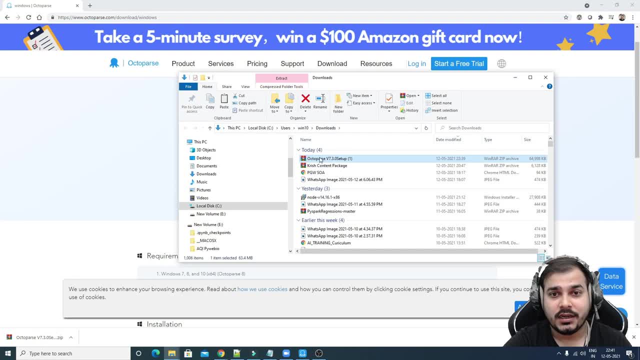 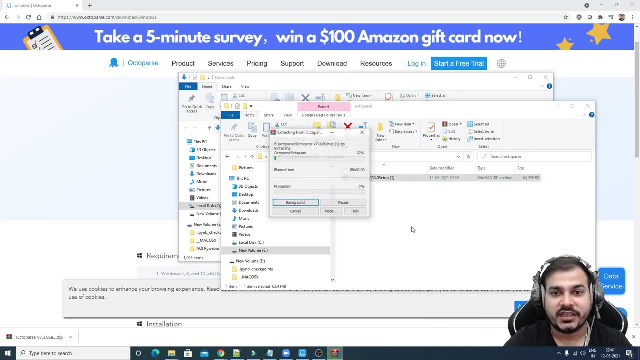 So, guys, after you download this particular zip file, make sure that you cut it off from here, paste it and create another folder of Octoparse. Probably you'll try to unzip it over here, So I'm going to extract it And once you extract it, you'll be able to find: 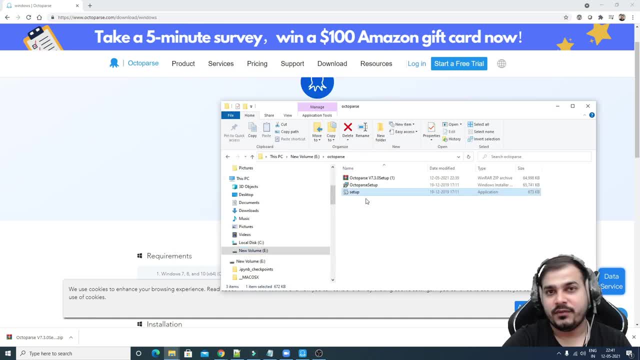 out this setup file. So after this, just double click the setup file and try to install it. It is just a simple process: Step by step, just try to install it. And once you install it, go and go to the start menu and just type Octoparse. 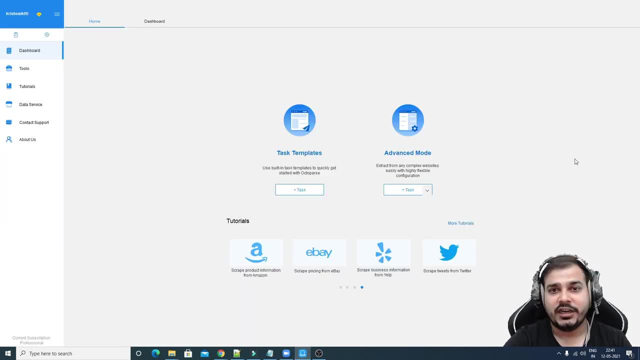 Now you will be able to find this particular tool that is actually downloaded right now. with the help of this particular tool, we are actually going to see how we can actually perform web scrapping in a very easy way without knowing any programming language, Right? So? 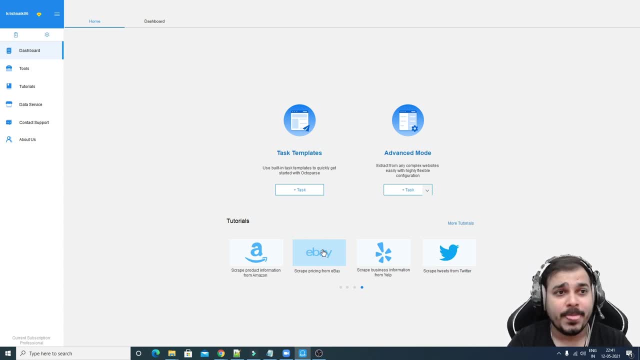 let's proceed and let's try to see what all options are actually there. Okay, So over here you'll be able to see there are a lot of different, different options. Here you have dashboard, here you have tools, So you also have different, different types of tools. 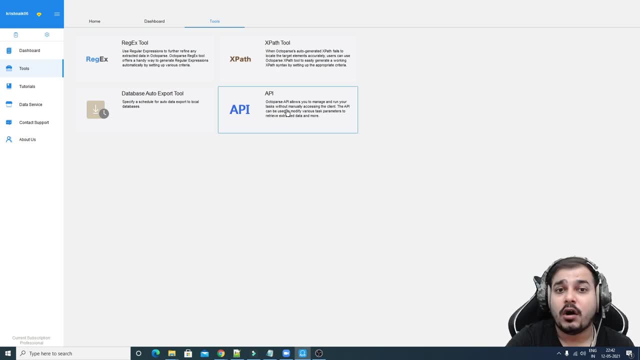 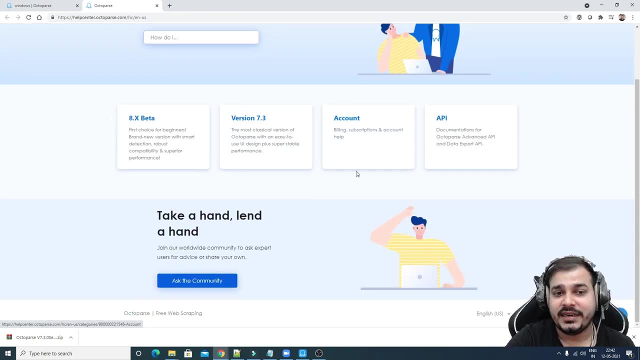 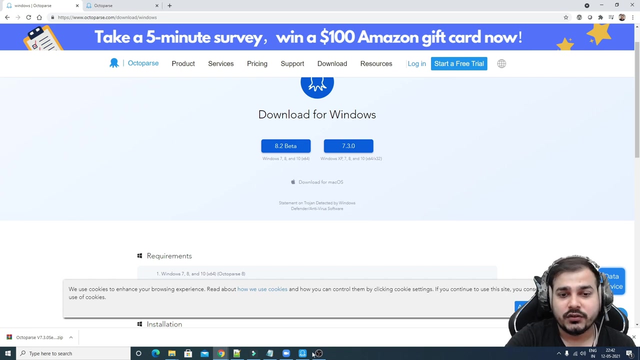 over here. You also have an option of creating Octoparse APIs, and then these are some of your tutorials, which you can actually watch in their website itself. you know so, with with respect to whatever version you are actually going ahead with, Okay, And then you'll also be able to. 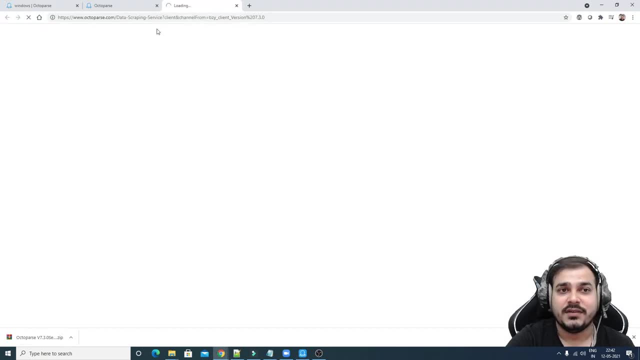 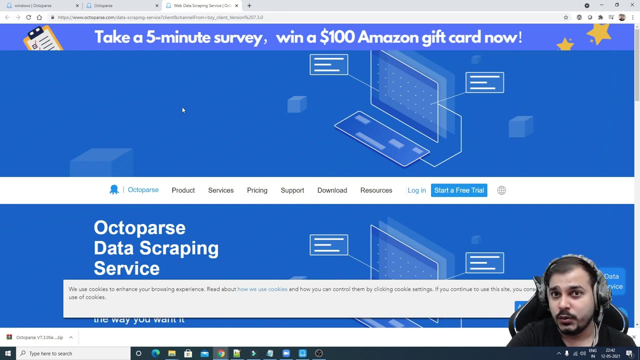 see if I try to open this here. you have something called a data service, data scrapping service, So this kind of facilities are also provided by this particular tool itself. that is Octoparse Right. So what we are going to do, I'm just going to go back with respect to this specific tool. 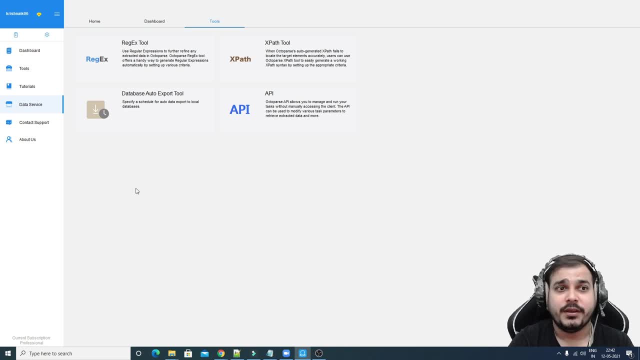 and we are trying to see that, what all things we can actually do from here. So let me just go back to my dashboard, or home Now. here you'll be able to see that there are some options with respect to task templates, and there is also an option with respect to advanced. 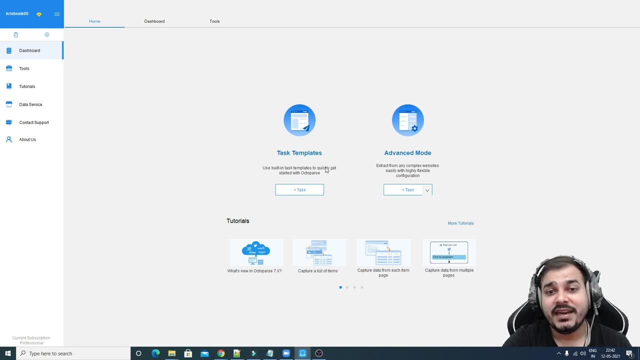 mode Now. task templates is nothing, but it provides you built in task templates to quickly get started with Octoparse. So if you just click over here here you'll be able to find various task templates, Right With different different websites. it's all together Like you will be having an option. 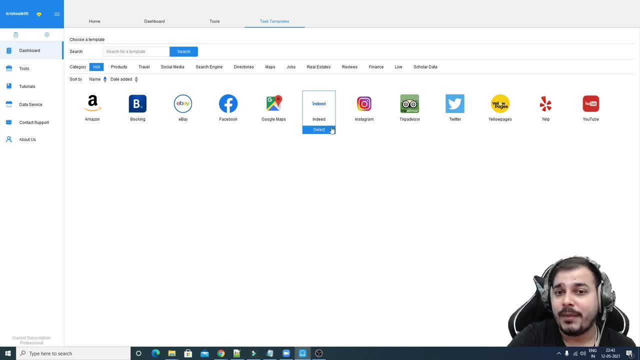 with respect to Amazon, booking, eBay, Facebook, Google maps, indeed Instagram, TripAdvisor, Twitter, yellow pages, Yelp and YouTube. So a lot of different, different products are there here. Also, you can see different, different categories, Suppose, if I go, and 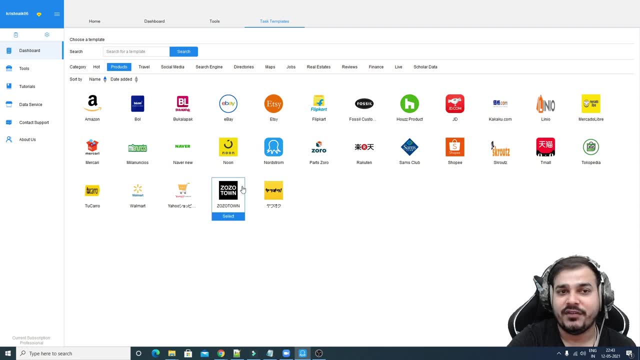 click on products, so here you'll be able to see more options with respect to different different products Here. if I go and click on travel the year, you'll be able to see so many products right Like TripAdvisor and all. 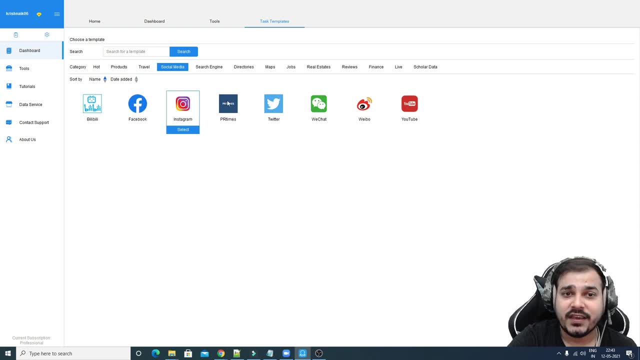 Yeah, You also have options with respect to social media, right Like Facebook, Instagram, Twitter, WeChat, YouTube, And then you also have options with respect to search engines. This is also pretty much amazing, because if you're able to extract the data from the search engine, 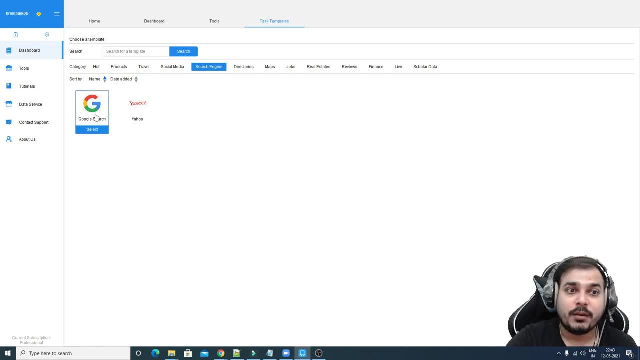 trust me, you'll be able to collect data in an amazing way. So you have options with respect to both Google and Yahoo. Then also you also have with respect to different, different maps. So here you can see Google maps also. You can actually explore some data. And these all are some fixed templates. you 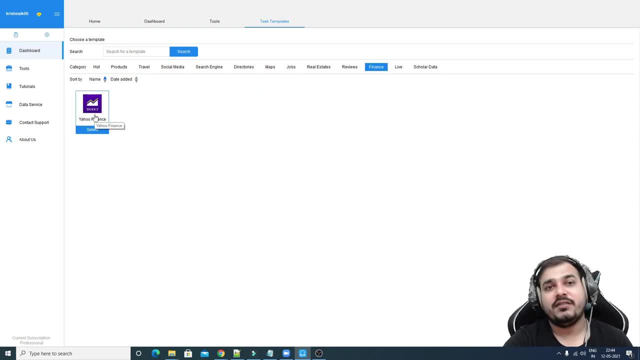 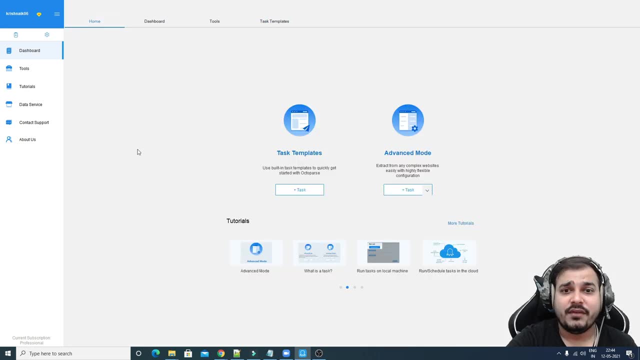 know. with respect to finance data Also, you have options to extract it from Yahoo finance And again, these all are possible just without any coding, So you don't have to worry about any coding as such. Now, if I go to back over here, you're also. you have something called an advanced mode Now in 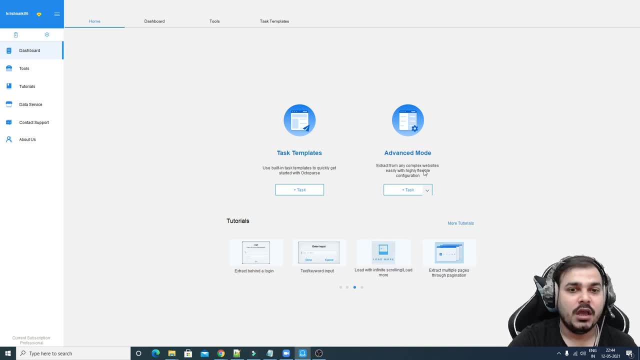 advanced mode, you'll see that extract from any complex website. Suppose you are you, you have a task where you need to web scrap from a very complex website, then you will be able to use this specific mode In this particular mode there. 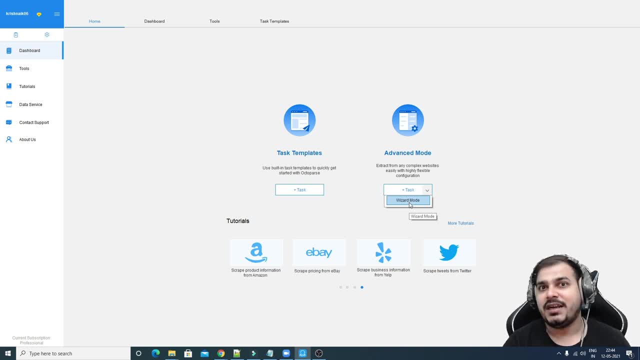 is something called a wizard mode. Now, with the help of this particular wizard mode, we'll try to scrap an amazonin- uh, you know, some web template. we'll try to extract some other details like titles, starts, cost of the product and some of the information like reviews and all, and we'll. 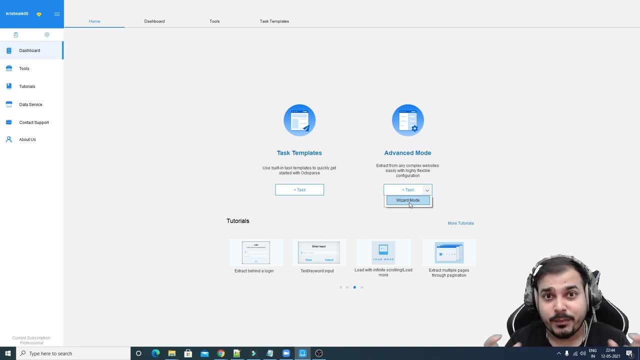 also make sure that how we can actually- uh, if there are multiple pagination, that also we'll try to see that- how we can actually scrap those kind of data. so let's proceed and let's take an example with respect to amazonin website. so, guys, now i'm going to take an example with respect to 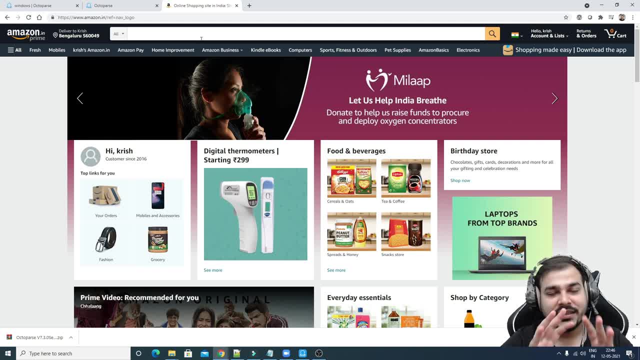 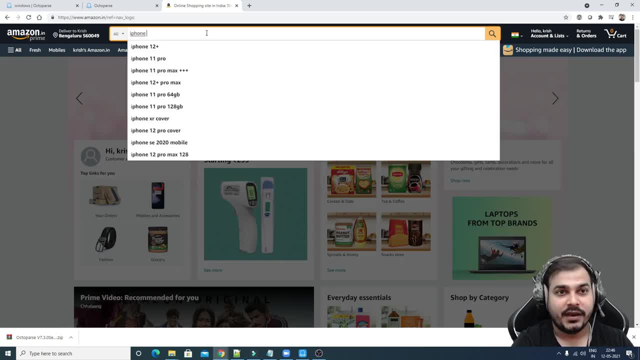 an amazonin website and we'll try to see how we can scrap most of the details with respect to various products. now suppose if i go and search for iphone 11 right now, when i search over here here, you'll be able to see a lot of products with respect to iphone. you'll be able to see some of 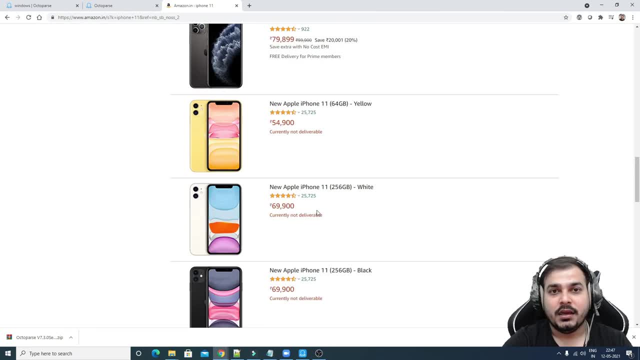 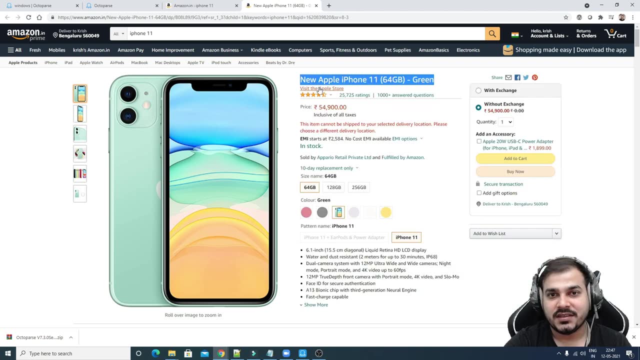 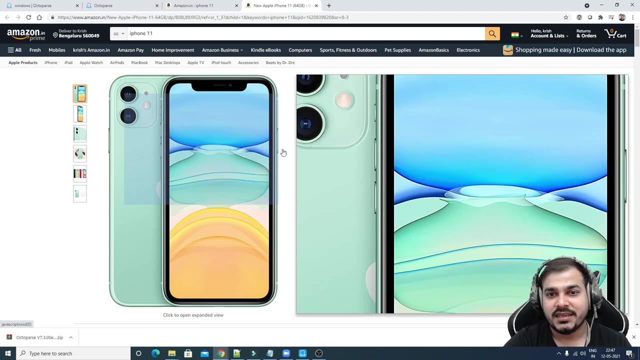 the information over here, like what all things are there and what all suppose. if you go and click a specific product here, you'll be able to see: this is your title name. this is your- uh, you know- brand name. probably. here is your ratings. how many number of ratings are there? what is the price? what are all? 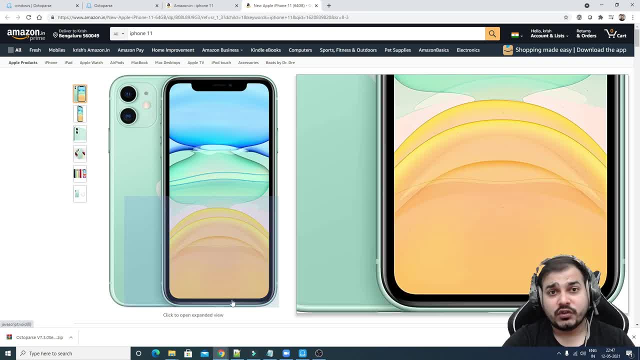 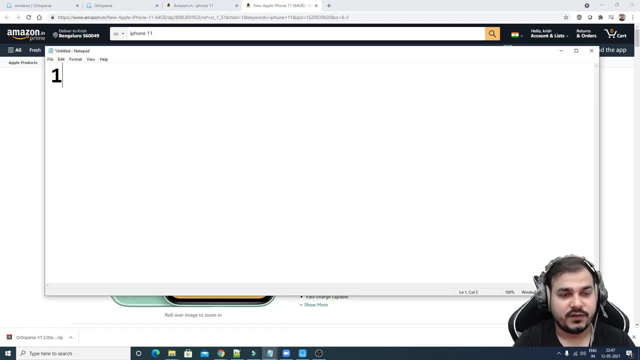 the other information. so if we really want to scrap this kind of website, we can basically follow five different steps. so let us see what all steps are there. so the first step: we will first of all go to the web page. right? so here we are. we go to the web page. second, we create something called as: 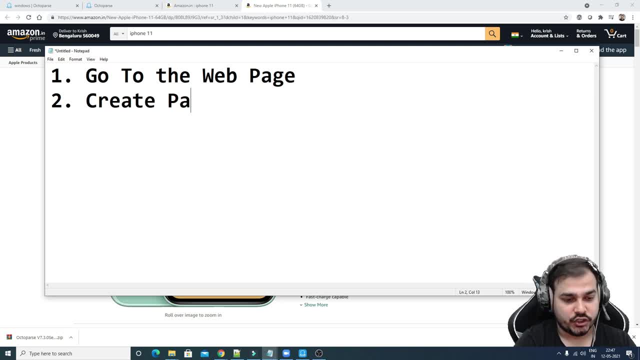 pagination. now why do we require pagination? let me just tell you, because i want to really scrap this kind of product details. so whatever search term i will be doing, probably i should be able to get the data. so if i go over here and just search for iphone 11, if i go on the bottom, 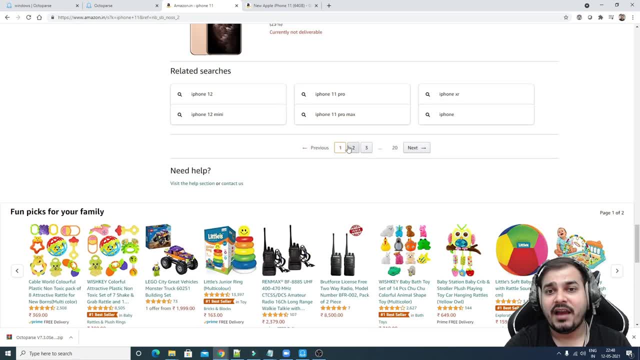 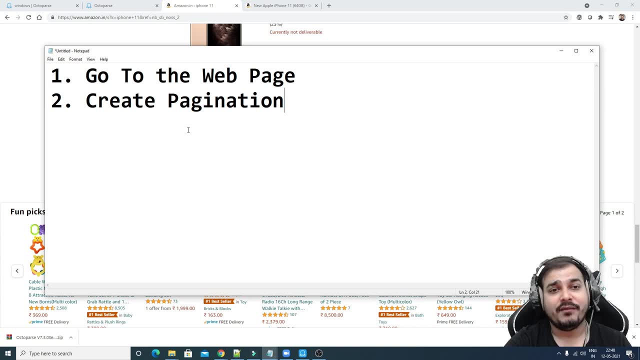 here you'll be able to see a lot of pagination and here also you have many, many products right. so we'll try to scrap this particular product with the help of this particular tool. so that is the reason why i have actually written create a page in nation in my second step. the third step is basically build a loop item. okay, so we are. 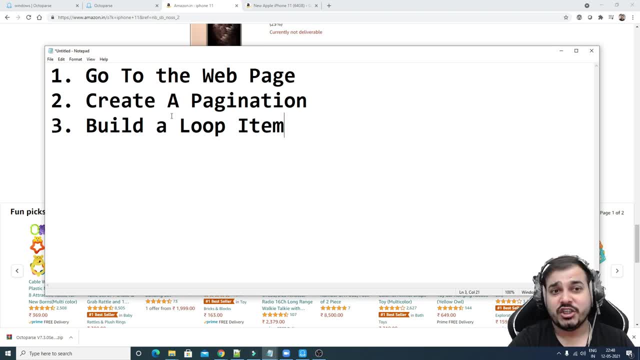 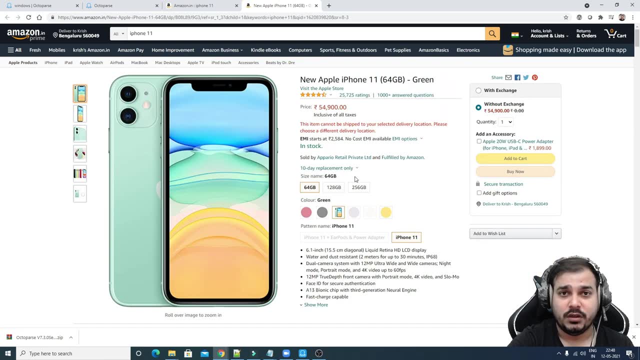 actually going to follow a loop light item because for that pagination we need to loop it again and again. try to extract all that particular details from this particular description page with respect to the products. so that is the probably the next step that we have to do: build a loop item. 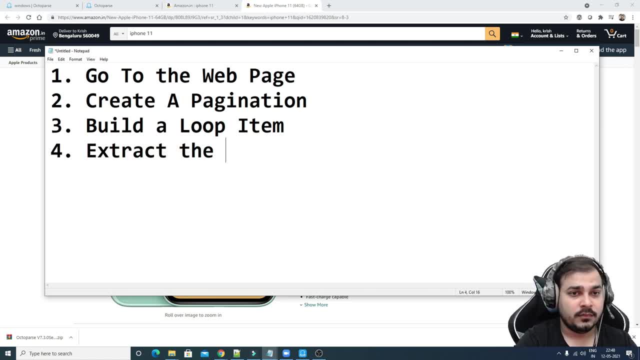 now coming to the fourth step, we need to extract the data in each and every description page, and then the Step five is basically run the task and get the data. So this is what we are actually going to do. First of all, we'll be having a web page. 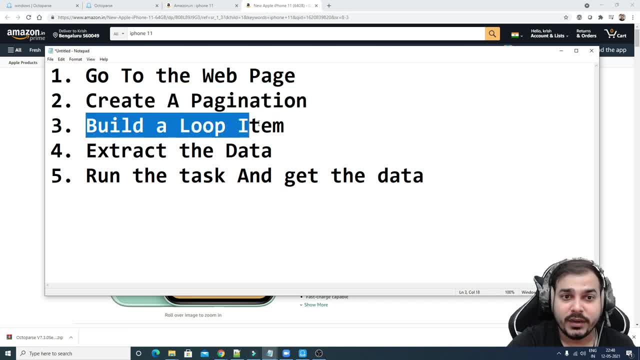 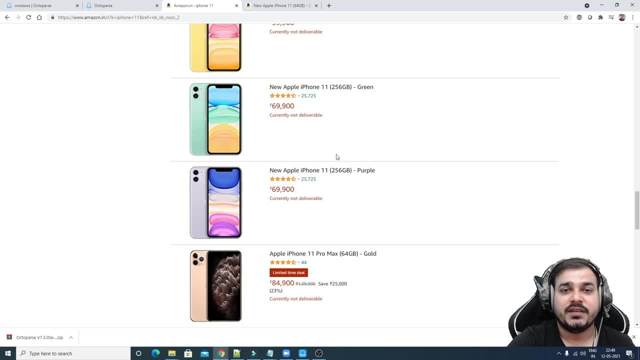 Then we really need to create a pagination And then we need to build a loop item. This loop item is basically to extract all these particular details from this description page of this specific products. And then the next step, which is my fourth step: 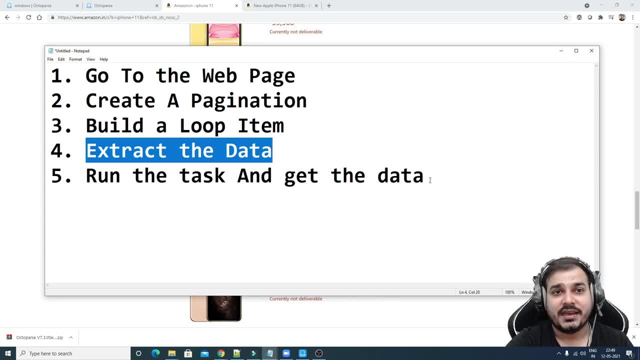 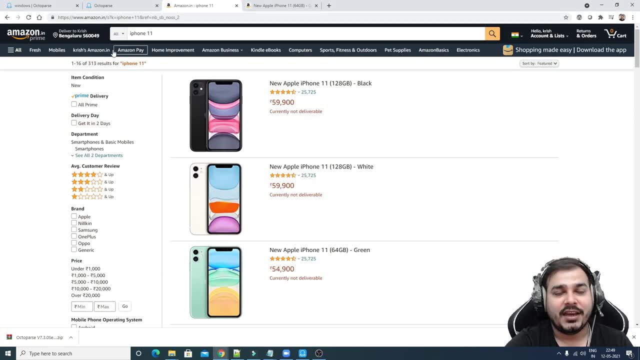 will be going to extract the data, And then we are going to run the task and get the data. So let's begin And let's go first of all to the web page I have. I'm there in my web page. I know I have to go and extract the data from here. 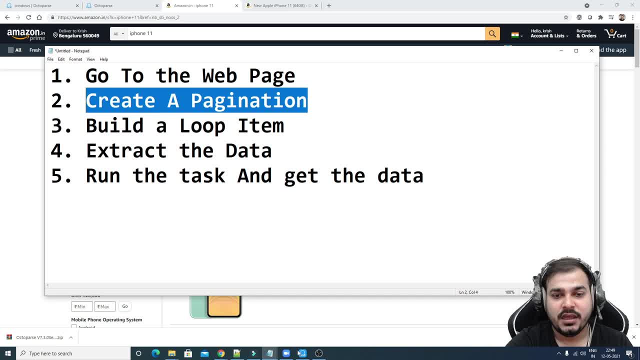 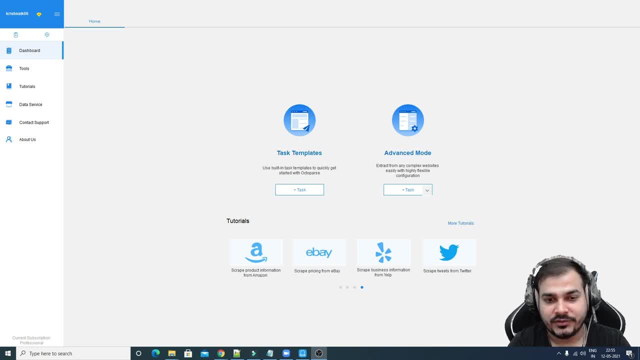 Now what we are going to do. we are going to see how we can create a pagination with this particular tool. So, guys, let's proceed And let's try to see that- how we can scrap an Amazonin website. I've already shown you this is my website details. 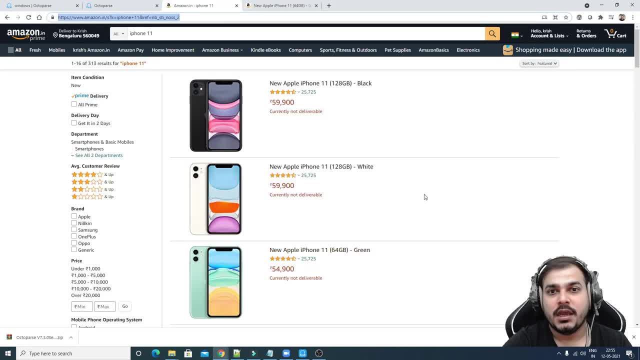 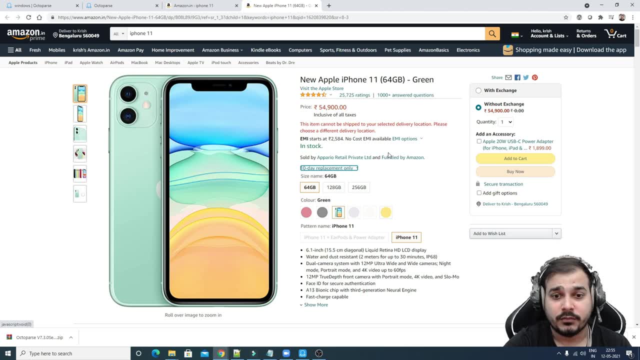 So here is my website details. Here you'll be able to see this. We will try To scrap this entire information, along with the description over here with respect to the product description information. So let me go over here And first of all, let me take the URL. 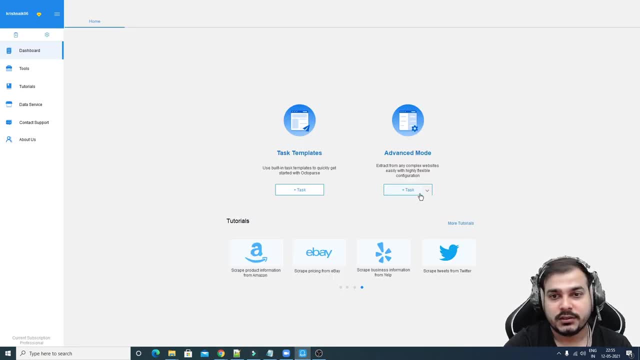 So I'm going to take the URL over here. Go to my Okta pass tool. I'm going to click on this particular advanced mode. Well, extract from any complex websites. Click on this plus here You'll be able to see the first option that you're getting. 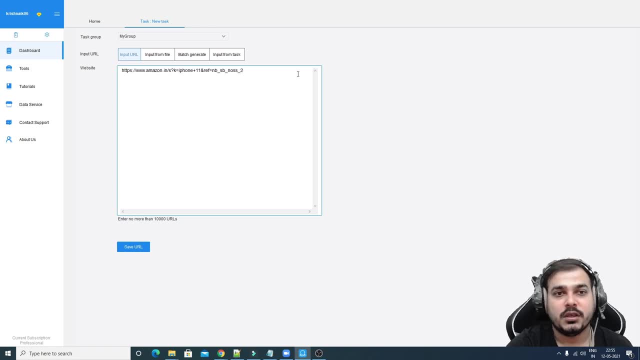 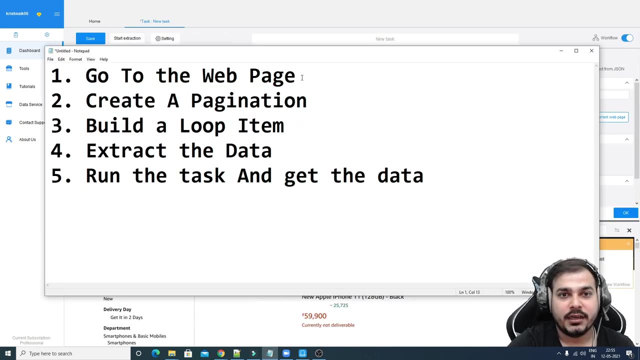 is to put the URL of the website. So I'm going to put the URL of the website over here And I'm going to click on this And I'm going to click on save URL. So this is the first step that I've actually written. 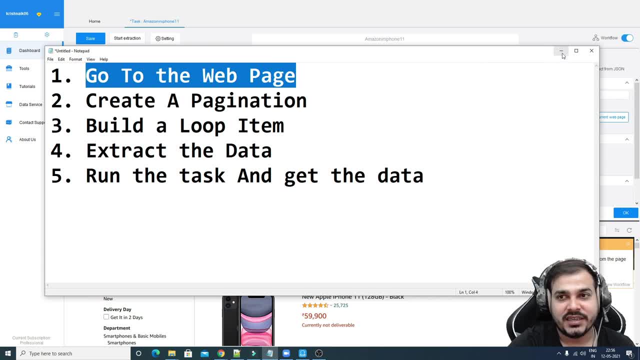 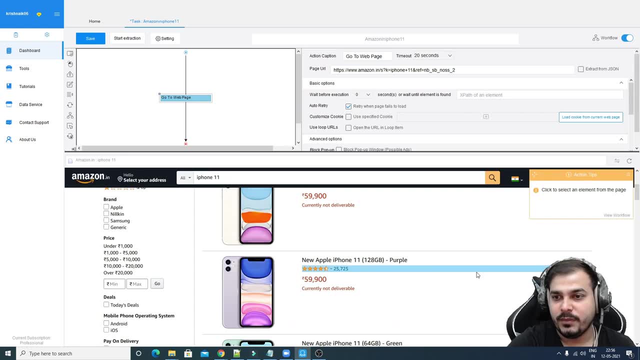 Go to the web page And, after going to the web page, get the URL and put it over here. Now, here you'll be able to see that this particular website will be visible below And you'll be able to find out everything. Now, coming back to this particular notebook, or notepad file, 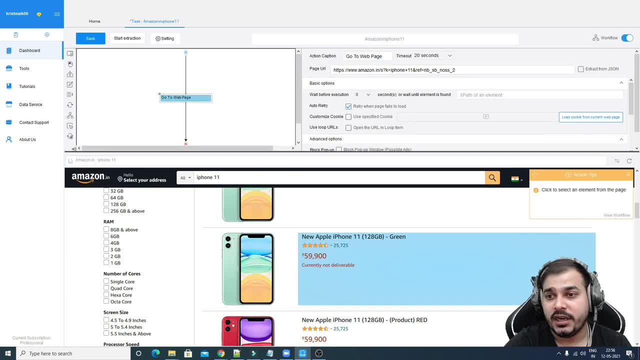 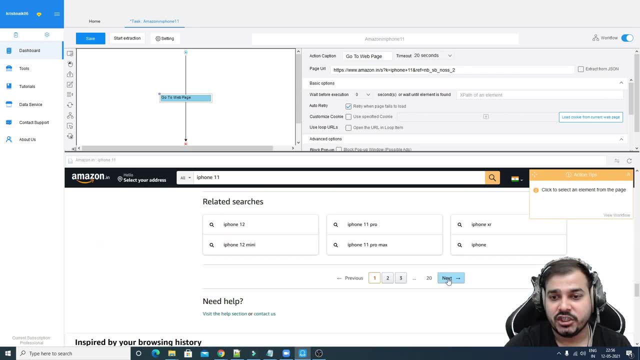 The second step is basically to create the pagination. Now, in order to create the pagination, go below, completely Right, And there will be an option in this particular page: Click on this particular pagination and just click over there in the next. When you click on next, you know you will be actually having an option saying that click. 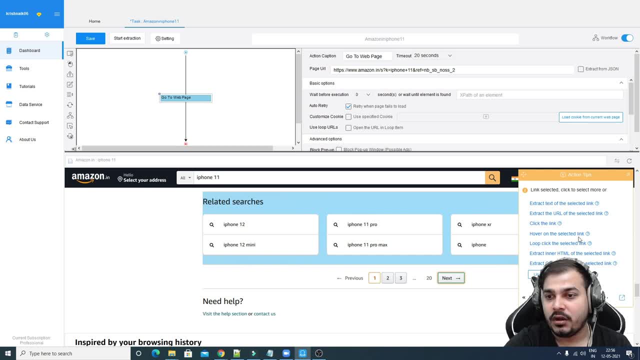 the link. See different different options. you'll be having over on the selected link And you'll also be having loop click. loop click the selected link. extract inner HTML of the selected link. So many of the different different options are there. 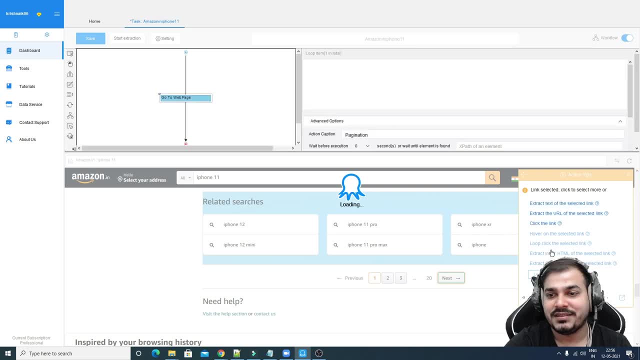 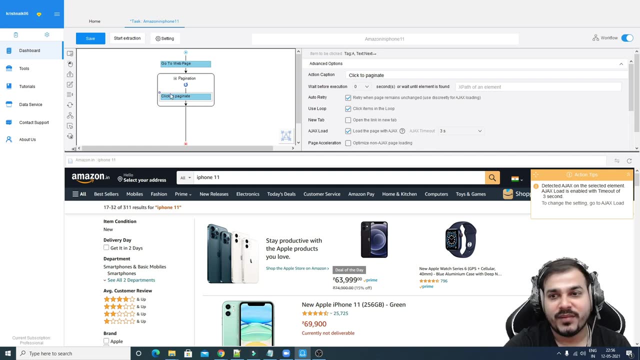 What we are going to do is that we are just going to click on this loop, click the selected link. When you do this, you will be able to see that The pagination will be getting created. So here you can see an option of pagination, and it also shows that it detect an Ajax on. 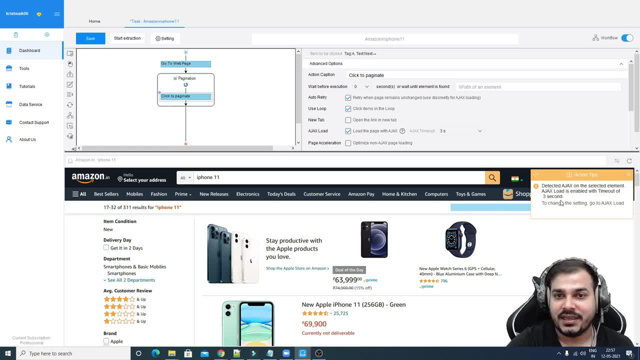 the selected element, Ajax load, is enabled with the time out of three seconds. You can also change that particular time out, but by default it actually takes somewhere around three seconds. If you want to change it, just go and click over here to change the setting. go to the. 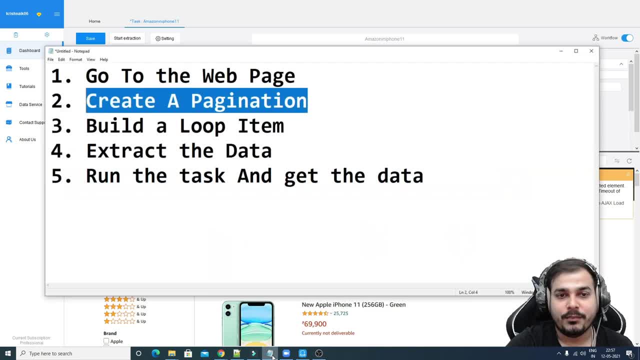 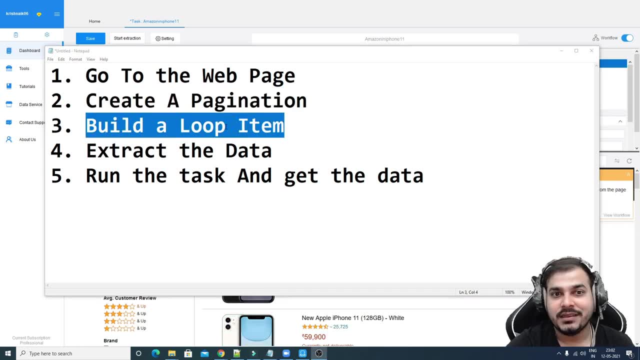 Ajax load Right. Pretty much simple. So we are completed. the second step, uh, that is creating a pagination. So, guys, Let's continue. the third step, that is building the loop item. Now, in order to build a loop item, first of all we will try to click on the go to web. 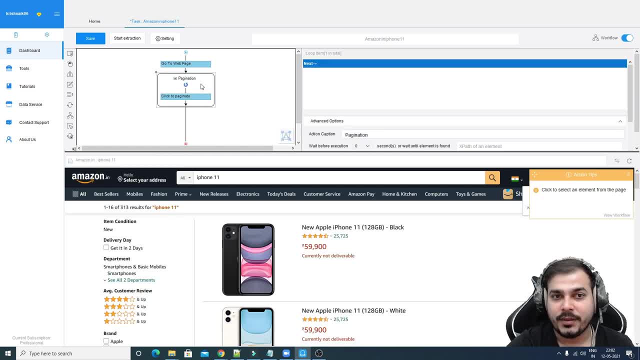 page, Okay, And over here you'll be able to see: let's click on pagination, pagination block entirely And after that just go and select any information over here. Let me just select the title of this particular product, Okay. 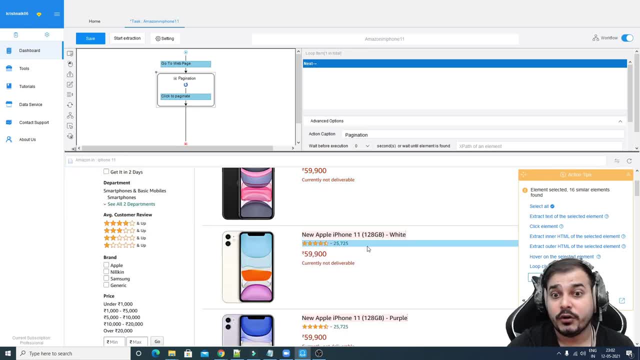 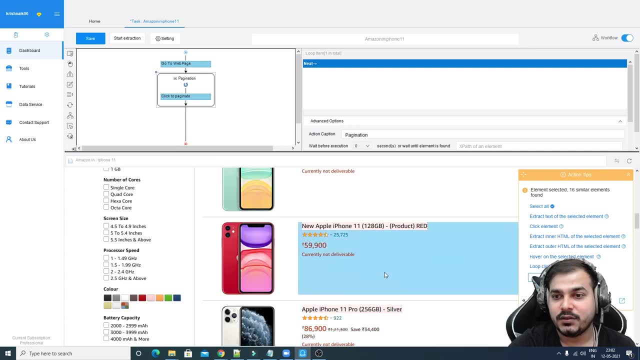 Now here, you'll be able to see that similar title. the octopus will be able to determine. the similar title is actually selected in all the Other products. right now, after selecting this, what we are going to do, I'm just going. 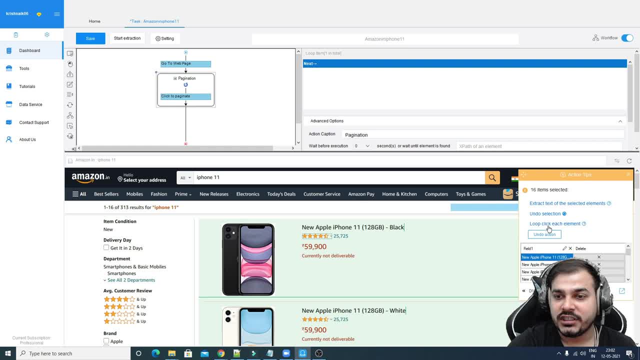 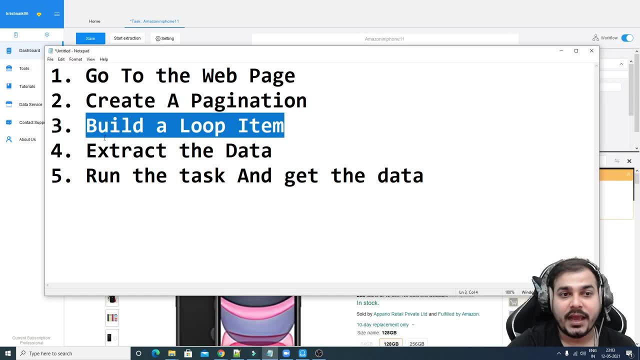 to click on select all. after selecting all, you just have to click on loop, click each event right Or each element. Sorry, Now here you'll be able to see that we are actually building a loop item. This loop item is basically for the product description page. 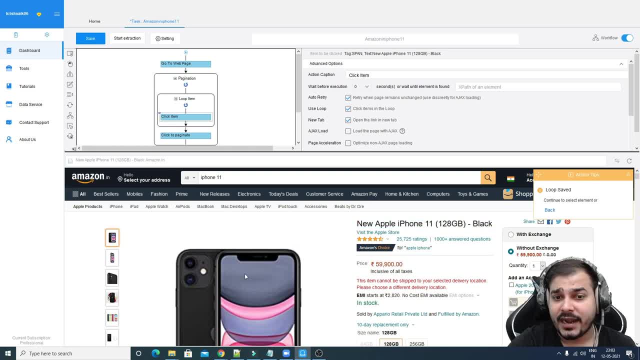 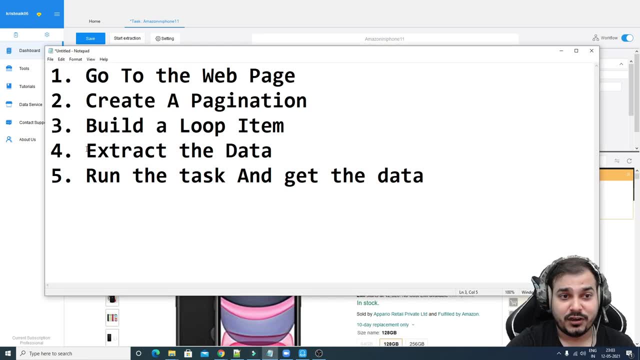 Now, when I clicked over there, loop over there here. you'll be able to see that we are into the product description page. Now, from this particular product description page, Which Which we will basically continue with the first four step, That is, extracting the data, 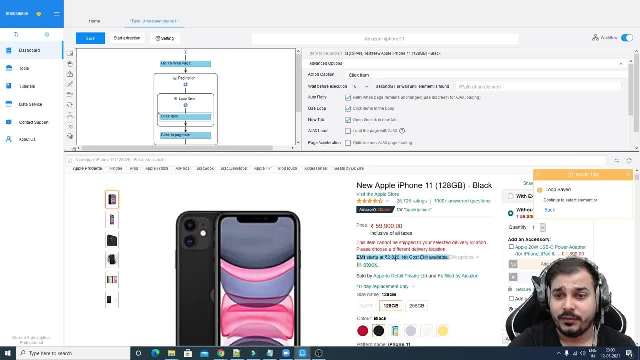 So what all data you actually want, we will be able to select from here. Now let me just consider first option over here. over here I've selected this, So from this I'm just going to extract the text of the selected elements. 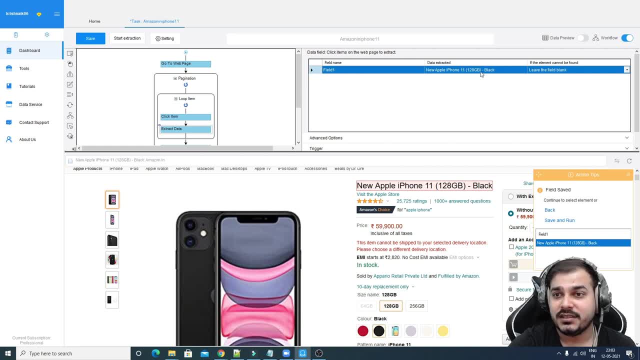 So let me just click over here. here You can see field one. This is basically selected here. I'm just going to say title. Okay, So this will basically be my title. Let's go and select the second element like: visit the Apple store. 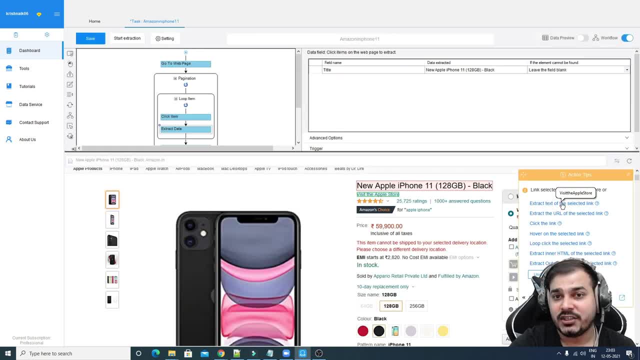 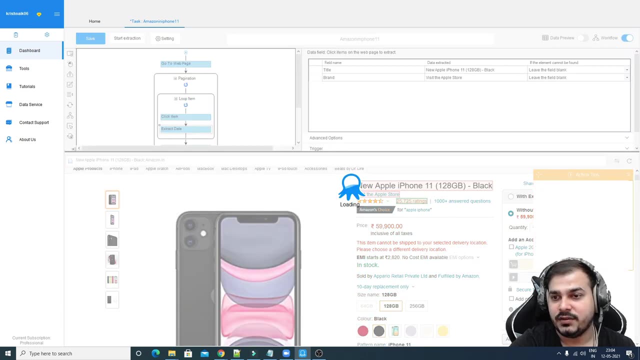 Now I'm going to just click on extract text of the selected link right again over here. So this will basically be my brand. This will be my brand over here. You can just select it as a brand. Okay, Now coming to the third one, which is this: specific ratings. 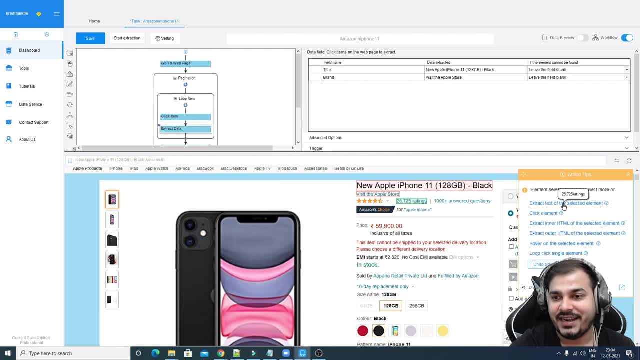 Okay. So here I'm just going to click on the text of the selected uh element. So let me just click over here and probably this will be my ratings: Okay, Ratings, Ratings, Ratings, Ratings, Ratings, Okay, And this will basically be my brand. 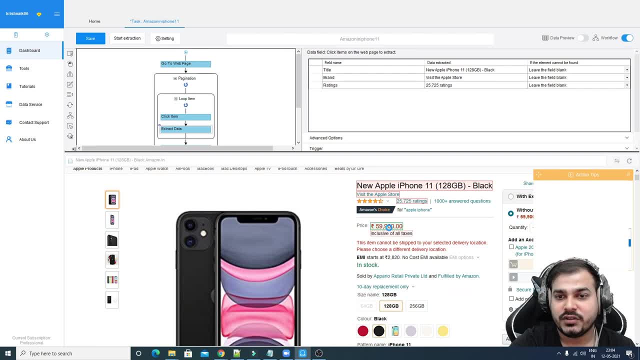 Okay, So all the elements has been selected over here. Probably I'll also select this because this is my price. So I'm just going to say extract text of the selected element. So this will be my price, and let me write this also. 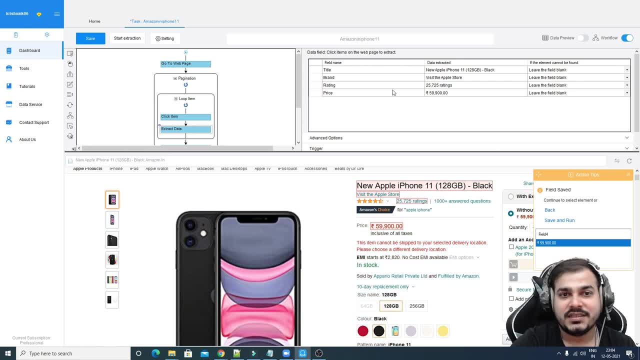 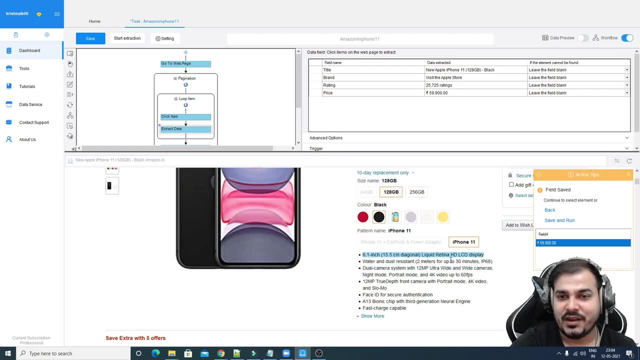 It will be my ratings. Okay, So this is all selected over here. I'm just going to take all this particular steps again. You can put up more information, This one like size, name and all. you can actually take out all this particular information. 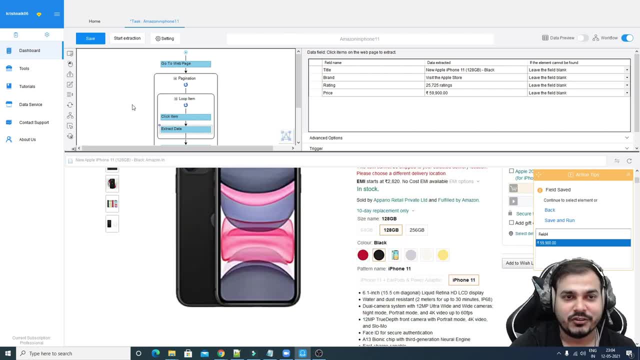 along with the description, if you want. but I really want to just focus onto this. And now what I'm going to do is that I'm just going to click on save. Okay, Once I save it now, I will just go and click on start extraction. 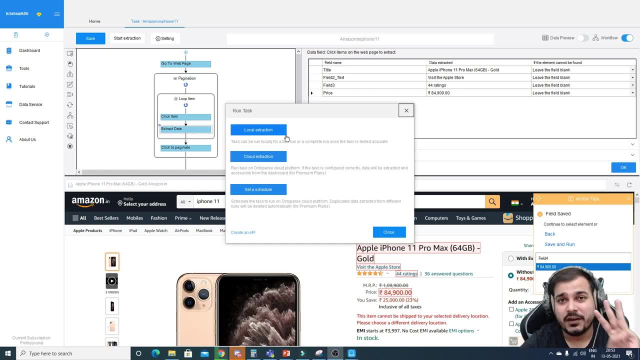 So, guys, when you're starting this extraction process, they are three main functionalities. One is local extraction, that you can run it in your local machine. The second one is called as cloud extraction. Now, this particular cloud extraction will help you to run the task on OctaPurse cloud. 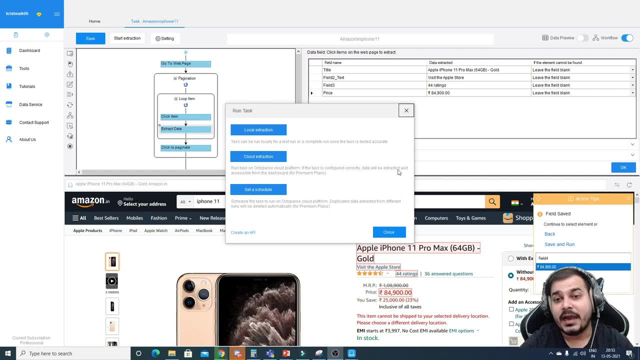 platform. If the task is configured correctly, data will be extracted and accessible from the dashboard for premium plans. And here if you're also planning to create an API, at that time you definitely have to use this cloud extraction. And third, one is basically setting a schedule like schedule: the task to run OctaPurse cloud. 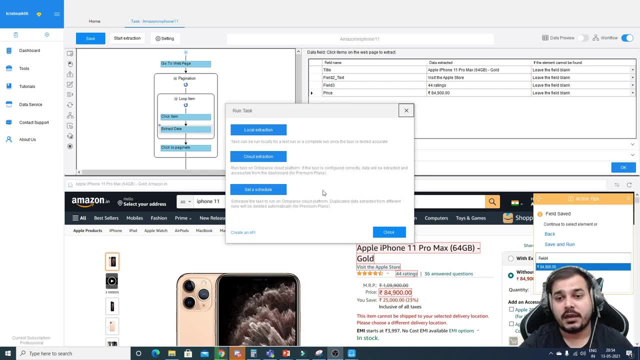 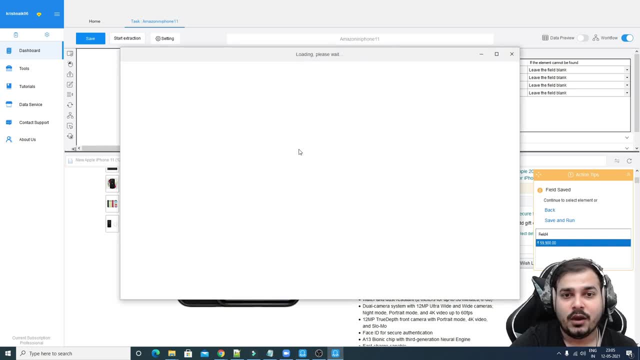 platform. So for this also, you probably have to use the OctaPurse cloud platform. Okay, So let's start, And let's first of all do with the local extraction. So I'm going to click over here and now. this will probably run. 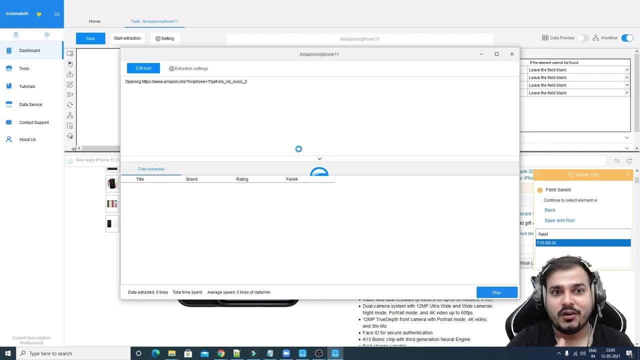 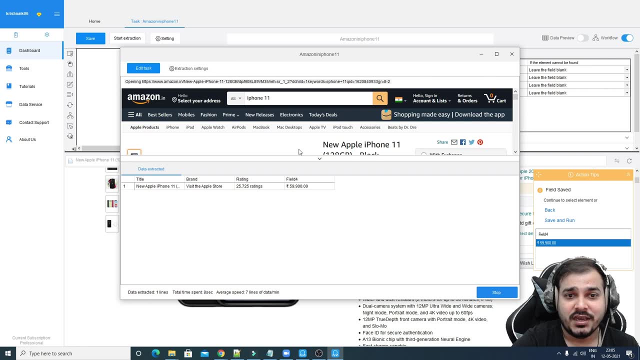 It will take some amount of time, you know, with respect to extracting all the details, because there you could find out 20 different pagination, right? That is the most important thing. So here you'll be able to see this information has come. new Apple phone title. visit the. 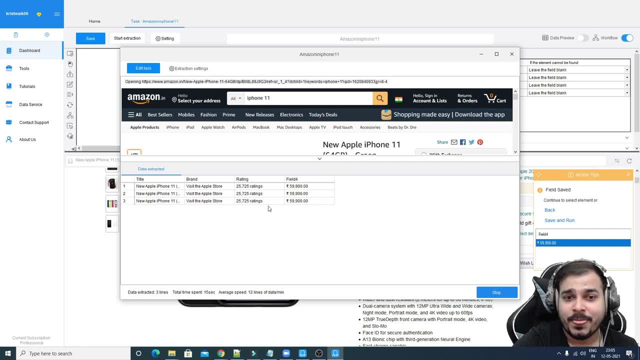 Apple store. The rating is this one, The price is this one, All the other information. you are actually getting it over here. Yes, Some of the items are repeated, guys, but here you'll be able to find out all the information. like back: white, purple, green, green product. 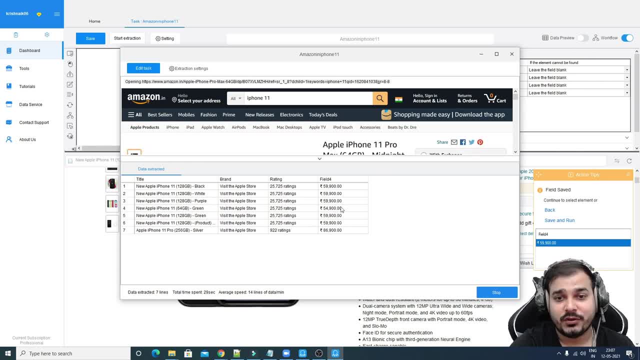 Here you are able to see all the things. The price is almost same. One is 54,900.. One is 86,900.. Then you also have this Apple iPhone 11 pro max. Here you are able to see all the details, right. 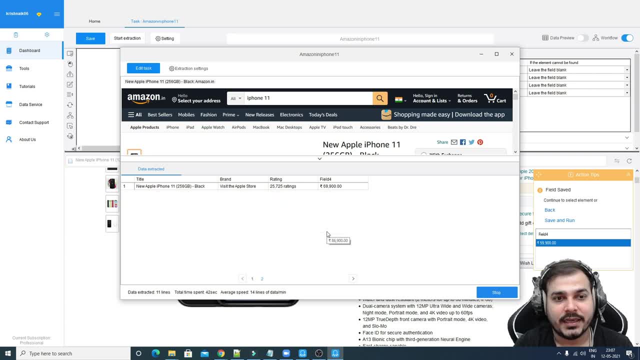 So now you are getting extracted. All the informations are basically getting extracted. Now, remember, guys, since they are multiple pagination, So Each and every page it will try to go into the product description page. try to pick up all the information and try to bring it. 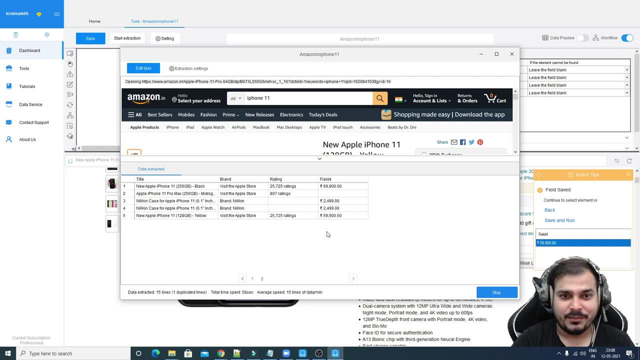 You know, if it is not able to bring some of the fields, then probably there may be multiple selected things over there or it is not able to determine. But yes, obviously when we are doing the data collection strategy- not all the data we usually 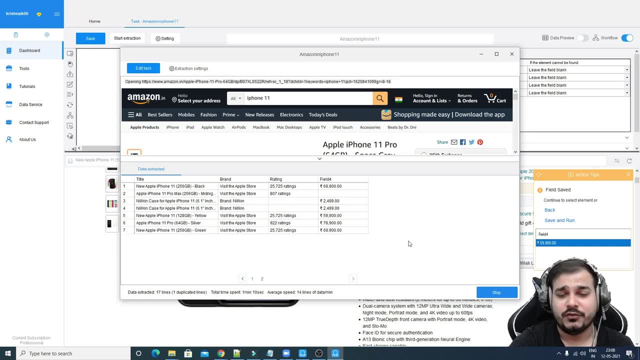 get right Sometime. we actually have some kind of problems over there. So probably this will take some time because, as you know, that we have somewhere around 20 plus pagination. So you can definitely go ahead with this particular process and you can basically select. 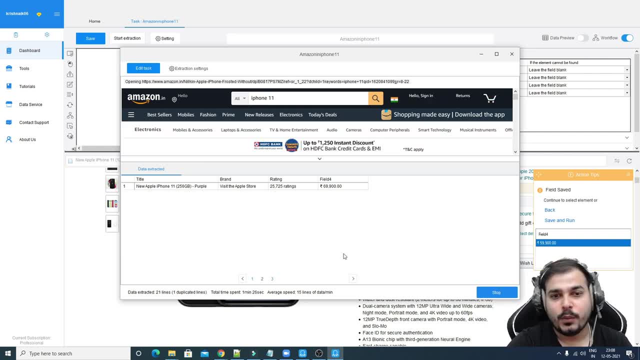 all the data. Now suppose I just want to stop it over here. You can see over here third pagination. it was able to get it from this. Suppose. if I stop it here, you'll be also able to see an option. Do you really want to stop this task? 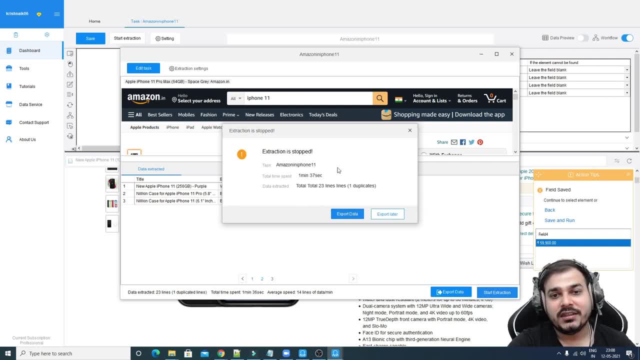 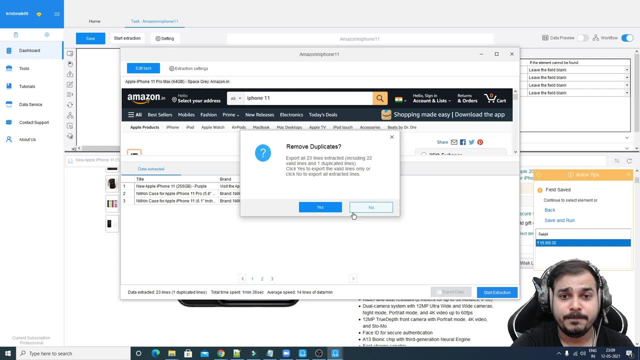 So I'll select them. Yes, Now you'll be able to see that on this number of seconds you are able to extract this many number data. Now, here you can actually export the data. Also, You can export data and here you'll be seeing exploiting, all 23 lines extracted, including. 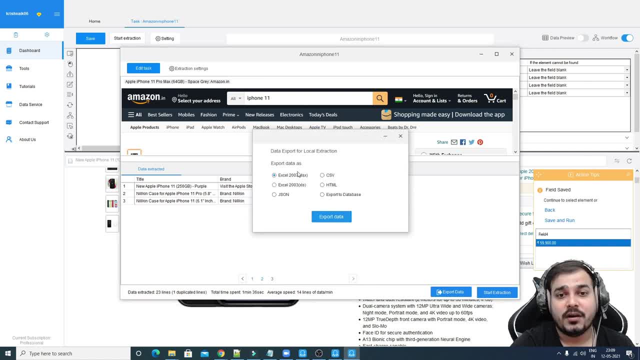 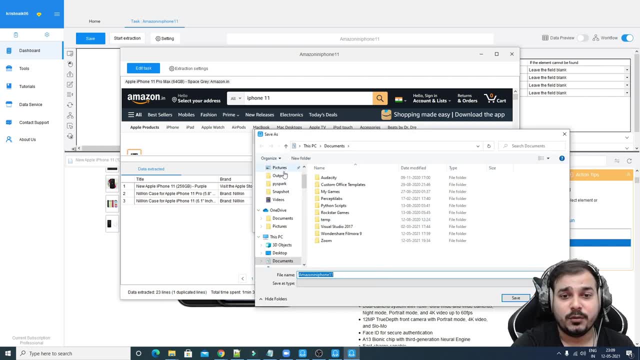 22 valid lines. I'll just select on Yes. Here you have a lot of options like Excel CSV. Probably I want to export the data in Excel CSV. or, Jason, I can actually do it. I'll just export the data and probably I'll just save it in my desktop. 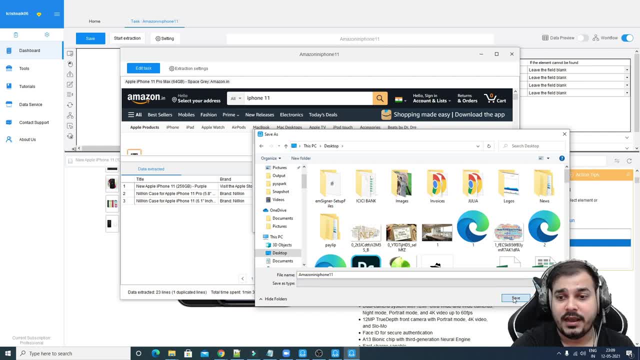 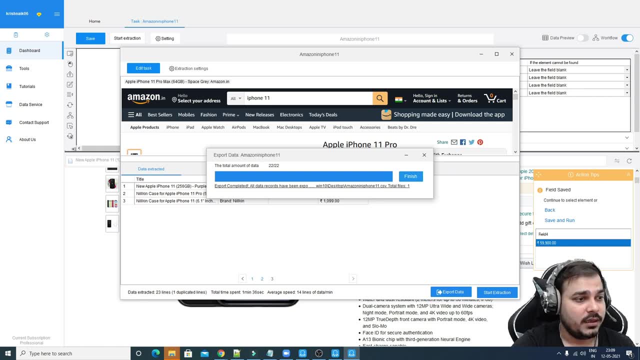 Okay, Save as Amazon dot uh in iPhone 11.. Now here you'll be able to see that the data has been exported. If I go and click this, you'll be. I will be able to open this particular CSV file. 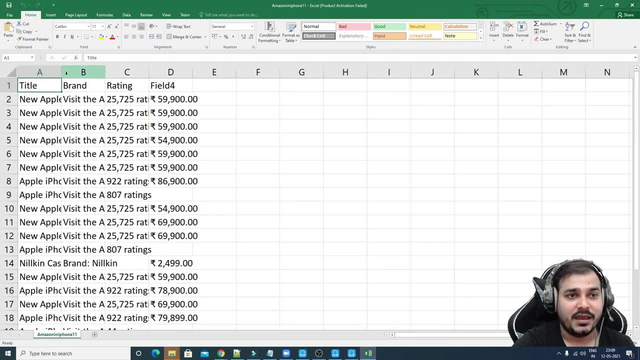 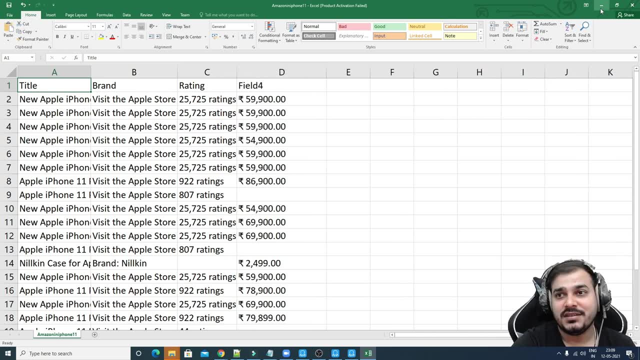 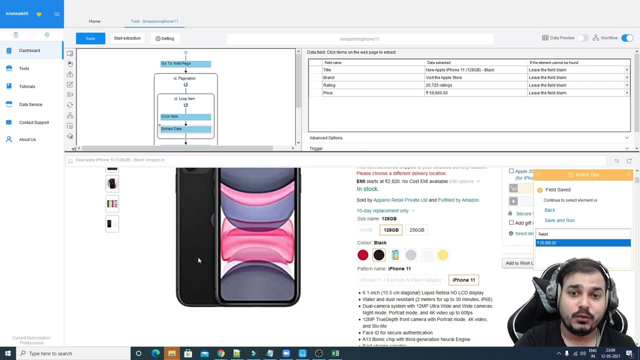 So here is my entire details with respect to the things that we have actually extracted. Again, web scrapping can be very, very handy, And here you could see that how amazing was this Octa purse tool because it was able to extract so many different, different pages right. 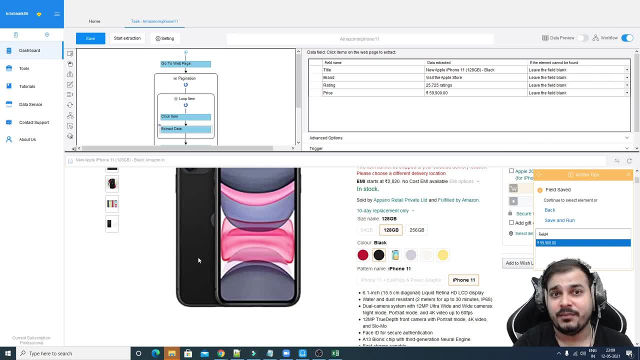 It was using that pagination building that specific item, and they were actually extracting all the details. This is with respect to Amazon Dot N guys. in the upcoming videos I'll also be making videos with respect to how you can extract flip card websites, yell websites, by using this specific technique. 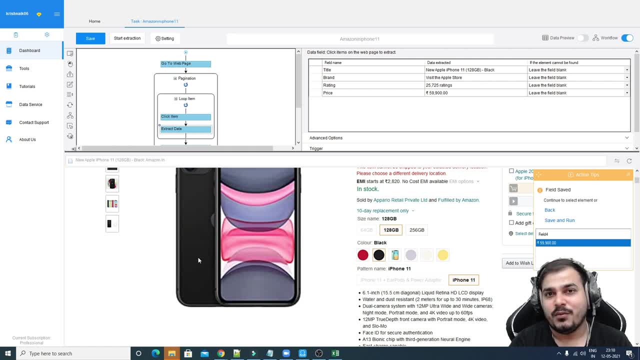 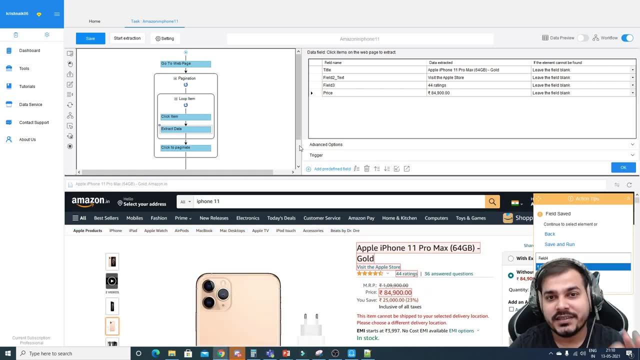 And I would also suggest you try out different, different uh websites altogether. Try to see, try to try YouTube channel also and try to get some information. Oh guys, here we are actually seeing that we are selecting each and every field. 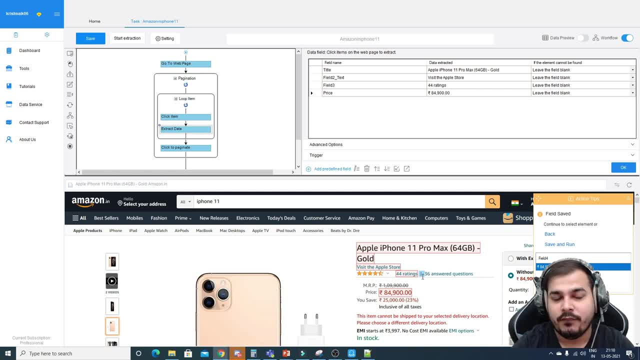 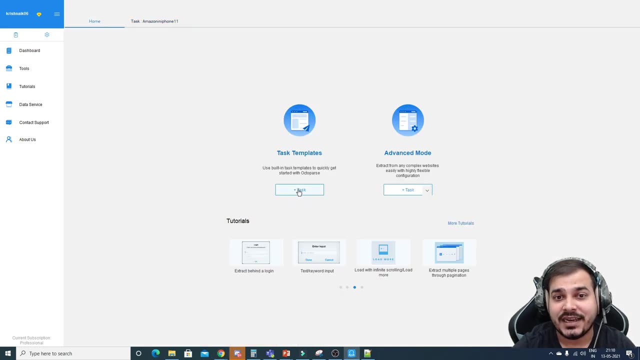 We are doing it manually. We are trying to extract this particular values from a complex website like Amazon Dot N And there may be chances because people who have not used this specific tool before, uh, they may miss some of the values. So what I would suggest is that you can go to the home over here and start selecting. 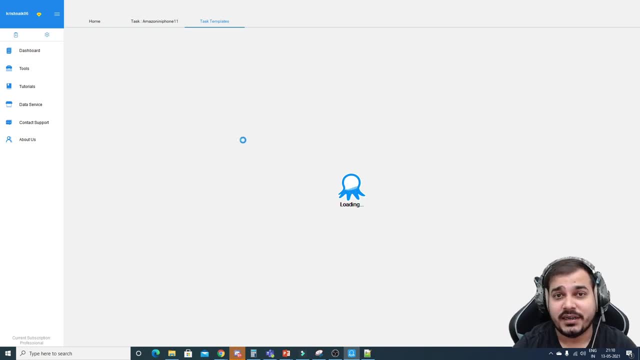 task templates and you can use different, different task templates. Now, what is task template with respect to different, different websites? They have a predefined templates. You know, if suppose, if I'm selecting Amazon, all the important information from that particular product page, product description page, uh will be able to extract it pretty much easily. 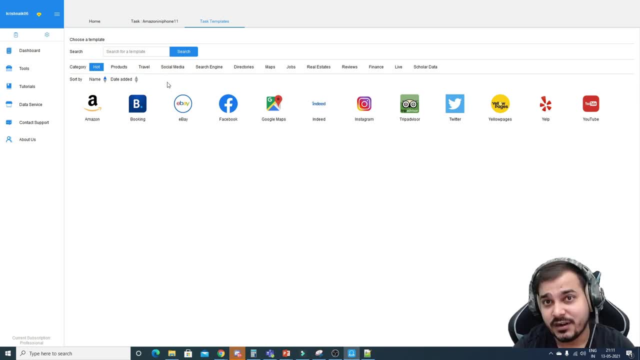 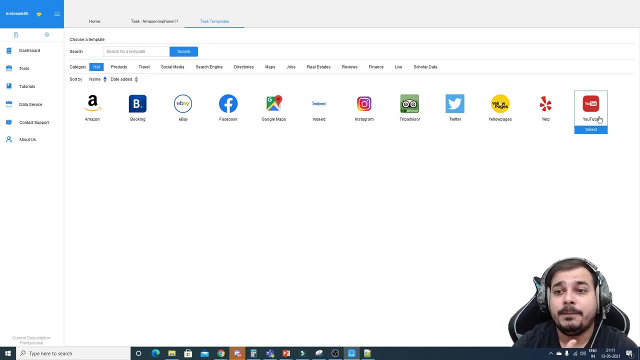 So definitely this, guys. you have a lot of options with respect to different different websites also, like eBay, Facebook, Google maps, Instagram, um and many more. Even YouTube is also there, and you can also check out with different different search. 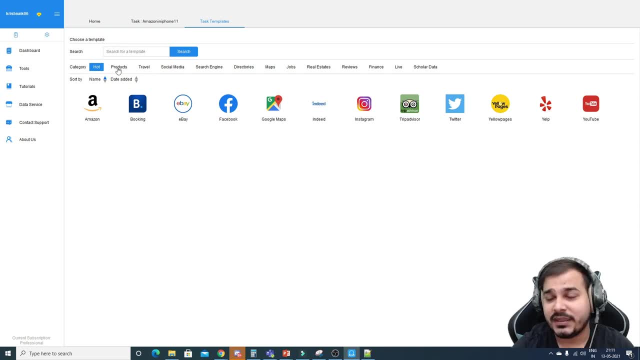 engines. So I would suggest that please try to use this kind of templates and try to see that how you're able to work along with it. But I hope you like this particular video again. Thank you, Octopause. This is an amazing tool for the professionals. 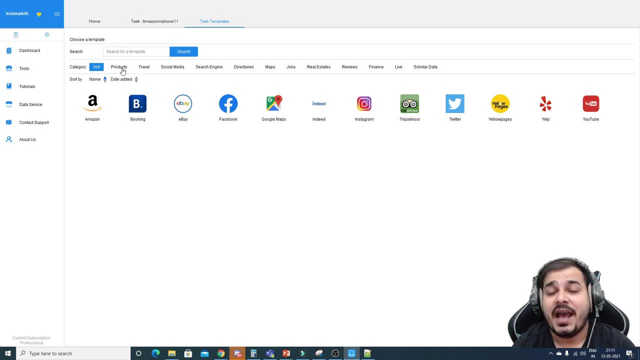 with respect to data science, for the data collection strategy, and it can be very, very much handy to all the people, because people from non-programming background can also use this specific tool. so i hope you like this particular video. please do subscribe the channel if you have. 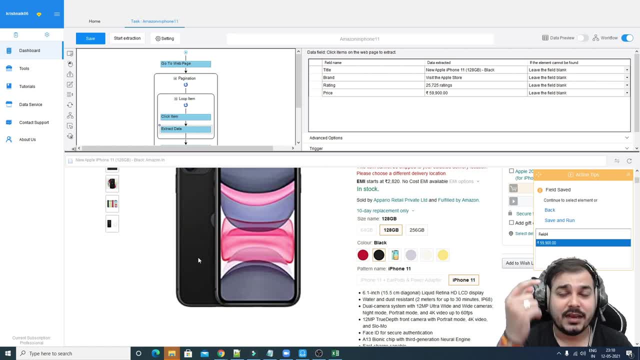 not already subscribed. and yes, guys, if you really want to use octopus, i provided the link in the description- download it and start using it, so i'll see you all in the next video. have a great day. thank you and all bye.